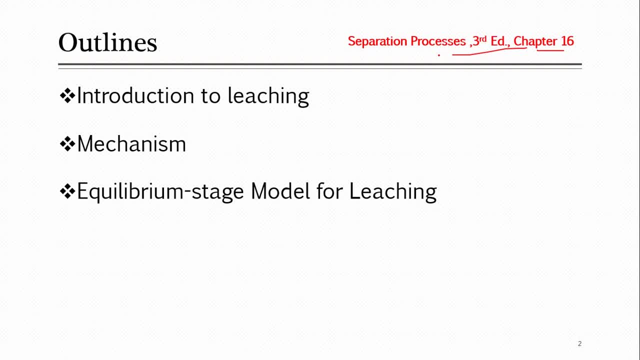 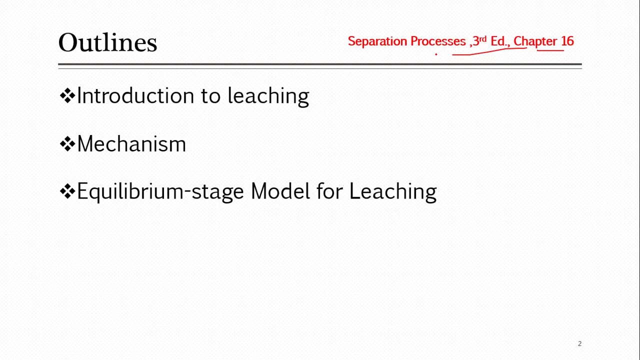 Fourth edition which we were already following throughout the semester. That didn't contain leaching topic. So leaching topic was included in only third edition. due to this, in the start of semester Maybe you remember I asked you to also mean have third edition because few topics we will cover from there. So this is the topic which we are going to study from the third edition Already when I uploaded the books in the start of the semester, So you have third edition there. If you didn't download, just go to the folder of books. 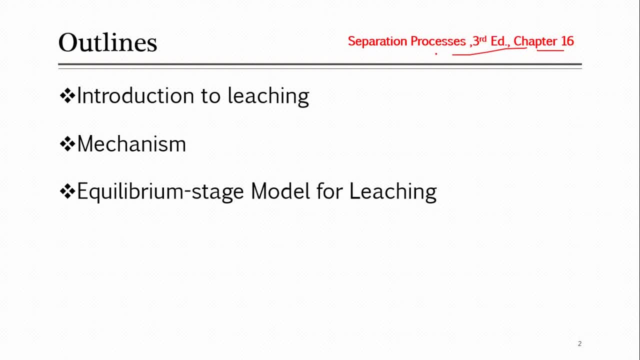 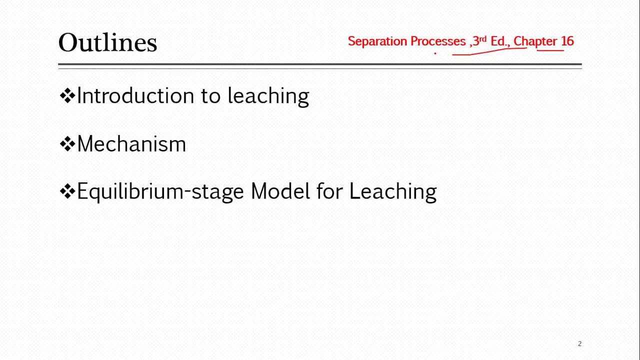 And get downloaded this third edition so that you can study the leaching topic from third edition. Before this, just to summarize, we discussed membrane separation and in membranes when we covered all those contents in four weeks that included basic introduction to the membrane, membrane material, membrane modules and then their application on industrial scale for various phenomena like reverse osmosis. 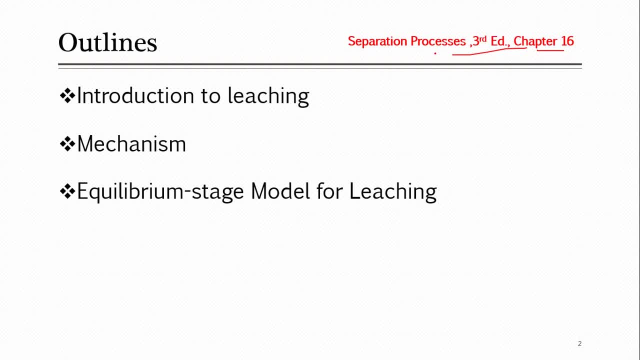 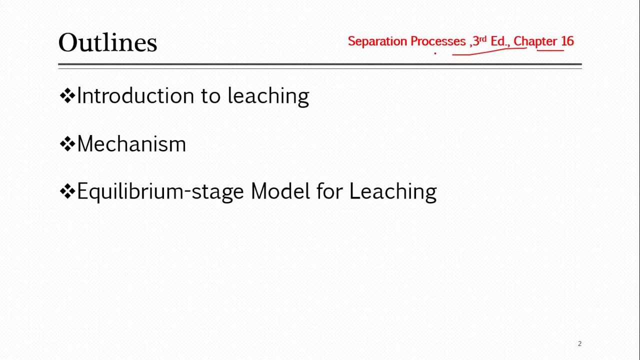 Membranes, then there were gas separation membranes and finally, in the last lecture, we discussed pervaporation membranes. Before that we discussed liquid-liquid extraction and before liquid-liquid extraction, actually absorption was detailed and discussed throughout seven weeks or eight weeks before midterm. So this last topic which we have to cover overall, 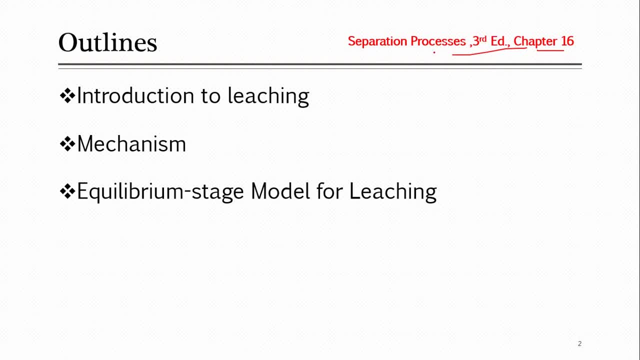 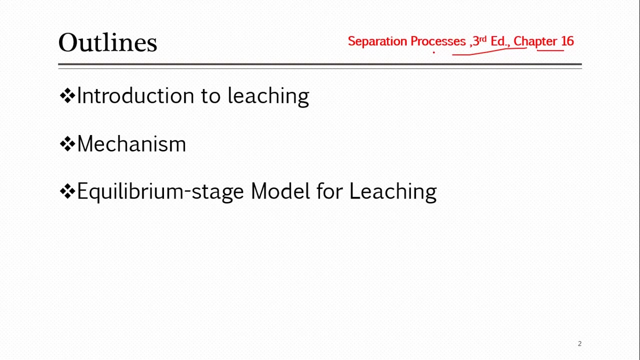 Here I am just going to cover major introduction and this equilibrium stage model, or they also called it sometime counter current washing model. So this we are going to cover, but only one thing which will be left. that was related to mass transfer phenomena in the leaching and the numerical stuff related to that which we can't cover, because this is the last lecture in which I will just introduce you with the leaching. 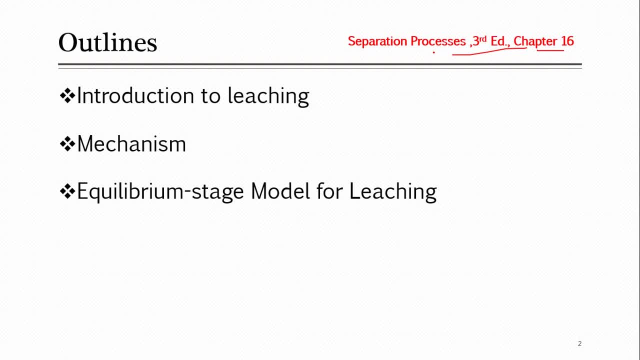 And we can't cover that only one topic. So overall, Alhamdulillah, we have done well throughout this pandemic and everything. Alhamdulillah, we may need to cover our syllabus, So let's start with this leaching. 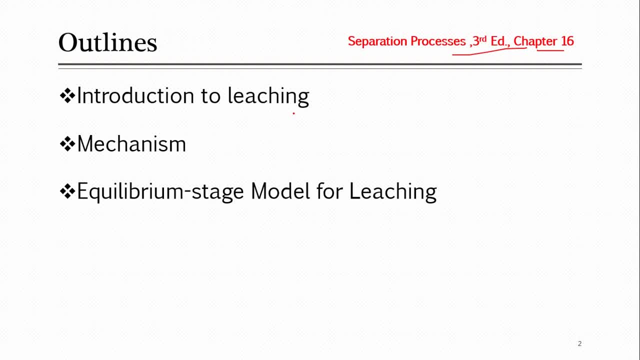 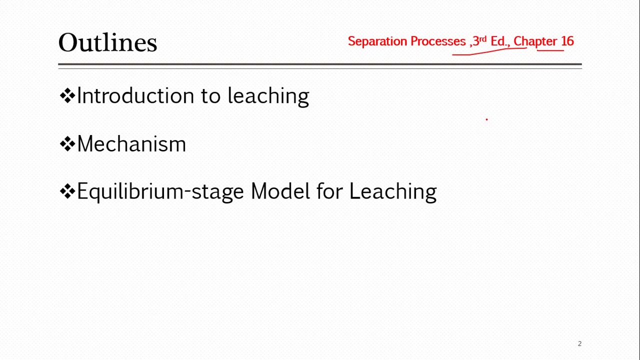 What is leaching or what is this solid liquid extraction? Before this you studied liquid-liquid extraction. So just to recall, liquid-liquid extraction actually involved two liquids. One liquid was Our feed and if you remember at that time, the liquid which was feed, that consist of two parts: one was carrier and other was means, some solute inside that feed and an external liquid. another liquid was introduced to the system and that was named as a solvent. 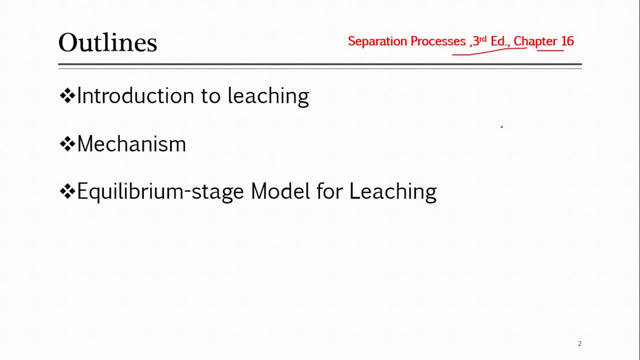 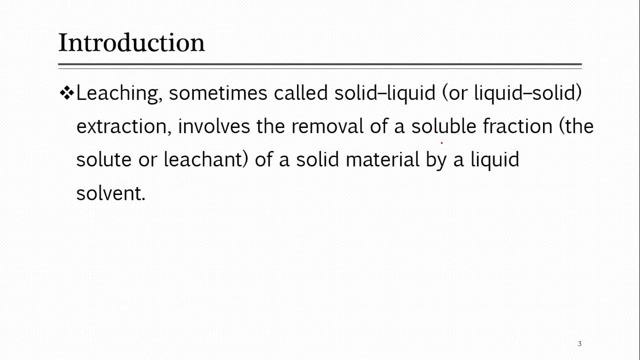 So that solvent actually extracted some components from this feed and those component were extracted which we were looking to be separated. So here, somehow same thing which we are going to have, that's the solid-liquid extraction. so inside this, let's look. what does this mean? leaching or sometime also referred as solid-liquid or liquid-solid mean- any name you can give it. extraction process involved the removal of soluble fraction of a solid material by a liquid solvent. 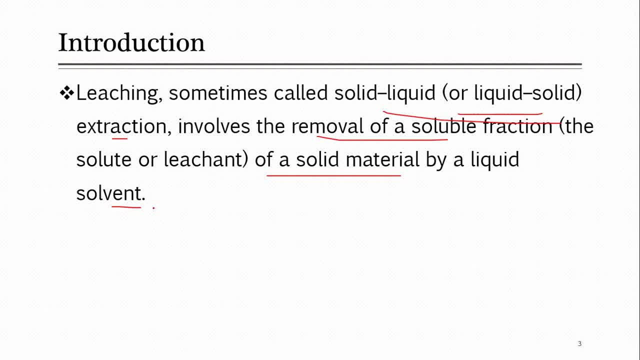 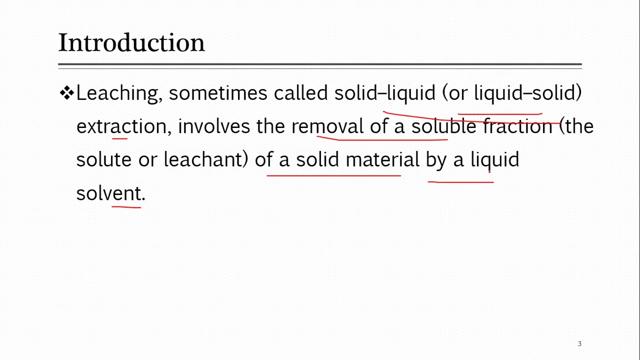 So it is somehow similar to the liquid-liquid extraction that in the liquid-liquid extraction you used to introduce some external solvent Or a liquid. so same here: you are introducing external solvent or a liquid and you are extracting, you are removing some part of the solid material or mean- removal of soluble fraction of solid material with the help of this liquid mean. if I compare it with the liquid-liquid extraction, there was one instead of solid that was liquid, which was existing in the form of feed. we used to call it as a feed. 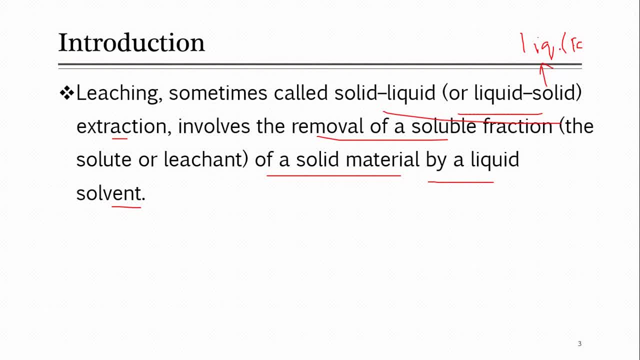 So at that time, that feed consisted Of one some carrier or solvent, as well, as some part was solute, which was recovered or which was extracted by another introduced liquid. so here same, instead of liquid in the liquid-solid extraction, you will have your feed as a solvent. 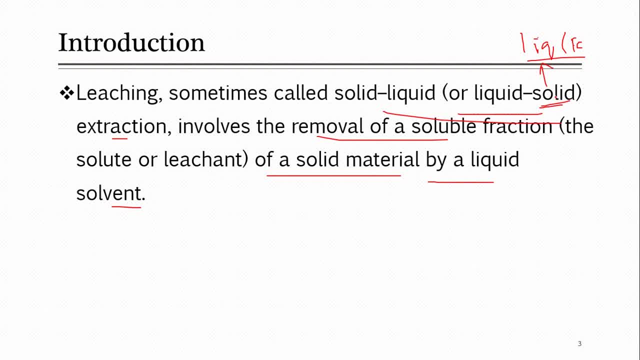 So that feed solid will contain two parts. some part will be like our required part which we want to extract, that's the solid-soluble fraction of that solid material. soluble means soluble in this. So instead of this you take some extra apartment for the afinic artıkic material, such that fecundated liquid. 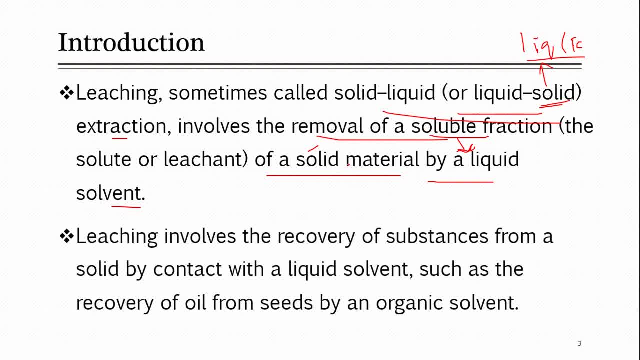 this liquid we are using as an extracting media so that some part is soluble in this while others are not soluble. So this leaching actually involved the recovery of substance from a solid, like in liquid-liquid extraction. you are recovery special … But here our feed is solvent. 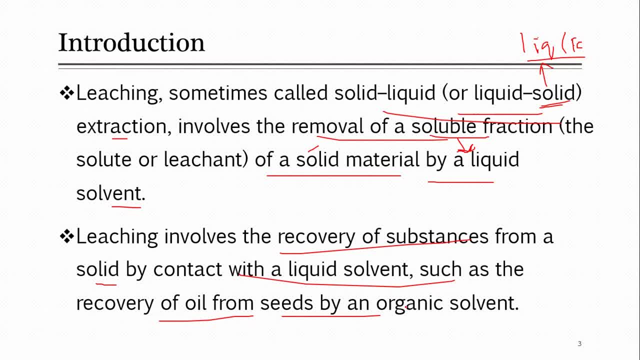 But here our feed is solvent. you are recovering some stance by organic solvent So we can recover various oils from seeds. mean, by using organic solvents, actually what these organic solvent will do: they will extract some oils. oils are also organic in nature and through from the seeds they will consist some cover. there are some. 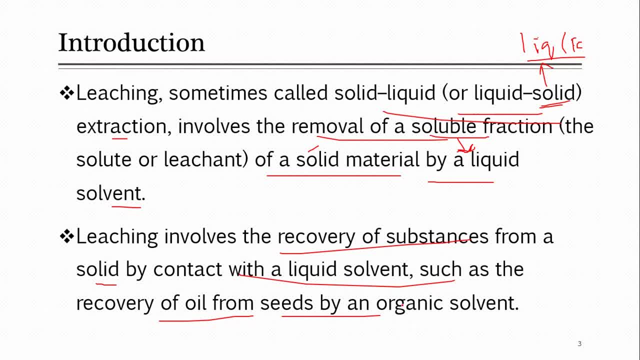 fibers and inside those fiber there will be some oil. So that is extracted with the help of some organic solvent and related to this extraction, or solid liquid extraction or leaching. I gave you one simple example of like tea beads or coffee beads, when you extract some. 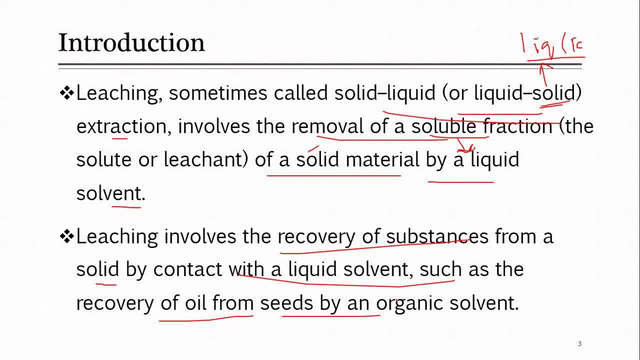 material from those coffee beads or tea beads or tea leaves in the hot water. So hot water now introduced, that is the liquid and we are extracting some material from tea leaves or tea beads. mean those tea beads are a solvent, So our solid or our feed, and out of those beads we extract some component or we will. 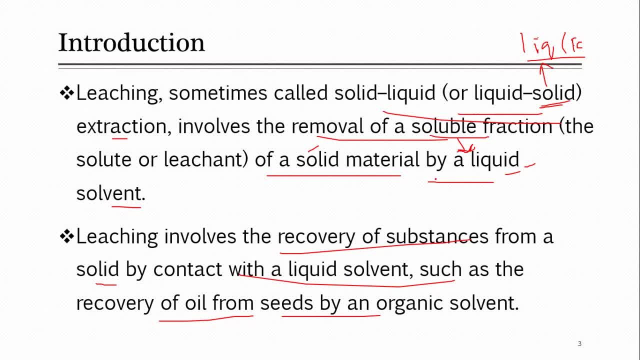 call it like soluble fraction of those components is extracted by hot water. So that is one example of the leaching I mean common, simple example of leaching which we already studied in the start of semester. So this was just definition or brief introduction of leaching. 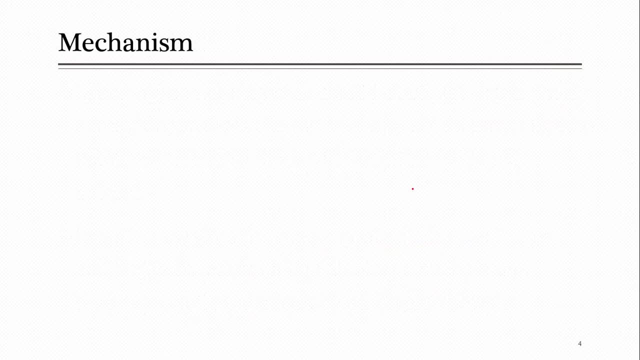 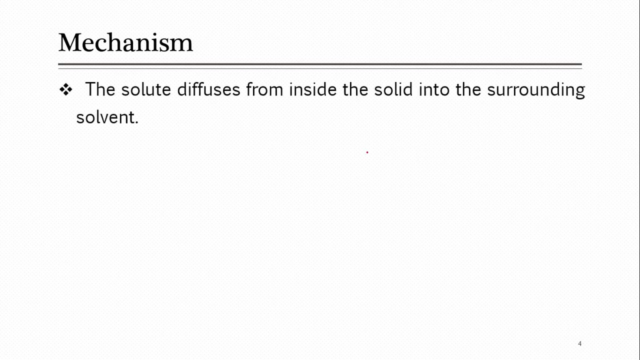 that, simply, it involved one solid and the liquid, and the purpose of liquid is to extract some parts of, I mean solid, and those parts which are extracted are actually soluble inside this liquid which is externally introduced. So let us look at the mechanism. how does this occur, or how? 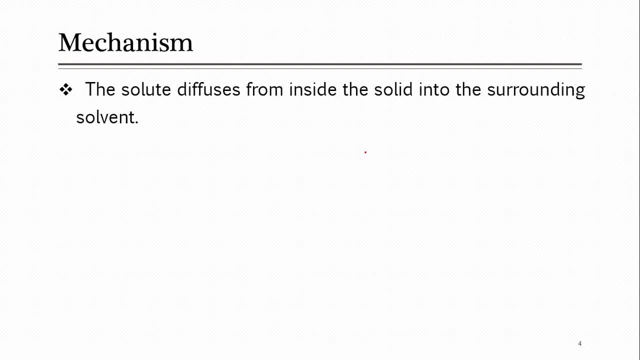 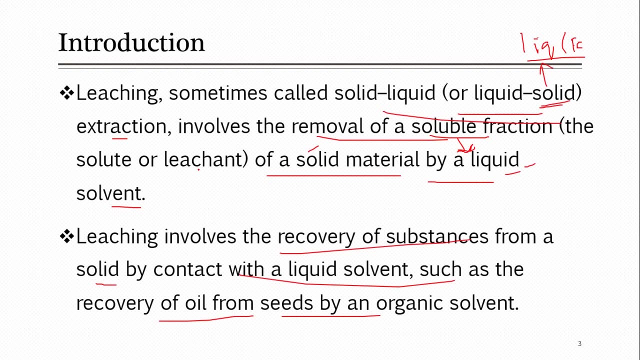 does this happen? The solute diffuses from inside the solid into the surrounding. by the way, this part is called solute, which we are removing, I mean here. he mentioned soluble fraction, which you are removing with the help of liquid is named as solute, or the leaching. 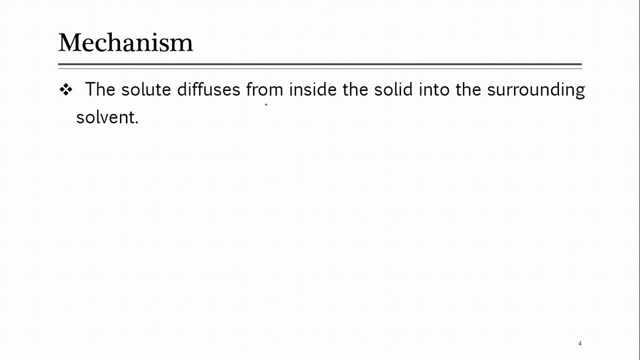 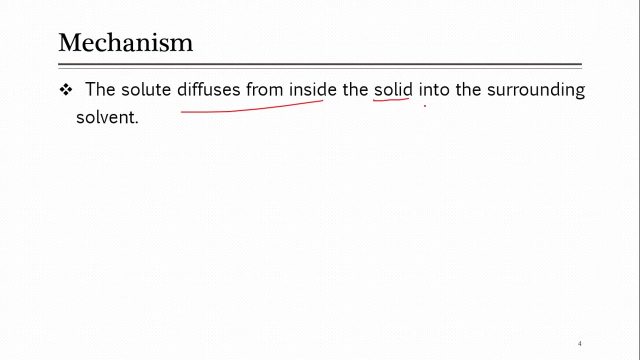 Solute or leaching that diffuses from inside the solid into the surrounding solvent When you add those solid inside some solvent, for example these tea leaves when you add them in the liquid water. So what happens? some part, some chemicals are extracted from those. 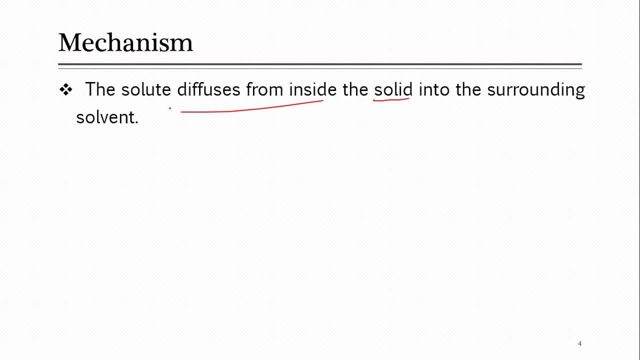 tea leaves and they are enter into the liquid solvent. So that is the. how does this occur? diffusion of those solute from inside the solid to the surrounding. Either the extracted And solids fraction mean here. when you are extracting something now, solid will be left. 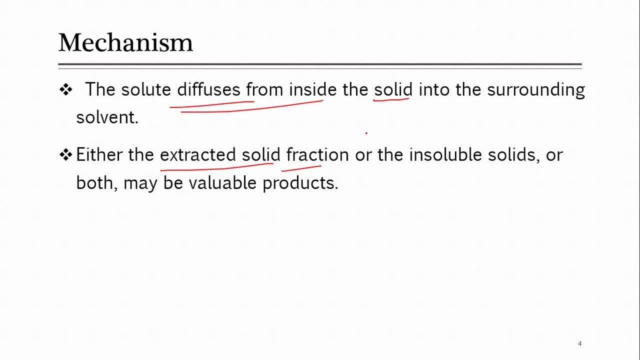 without those components. So sometime mean it depends either which of those is of our use. So either the extracted solid fraction or insoluble solid, or both may be valuable product, For example, when you are using this tea leaves, so at the end you just throw those tea leaves. 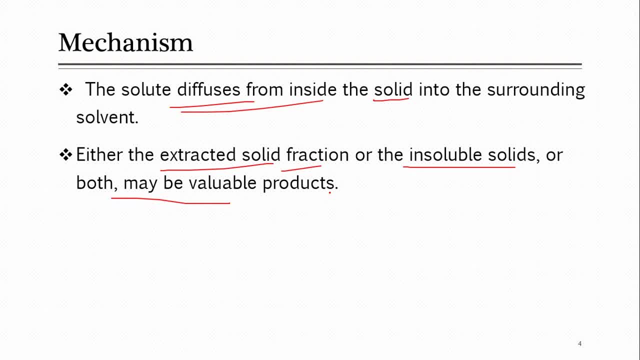 or tea beads, because they are of no use to you. You just mean, suppose, dip tea bag inside a cup of hot water and you extract the some part of this and then finally you just take away your mean tea bag and throw it away because that is of no use. 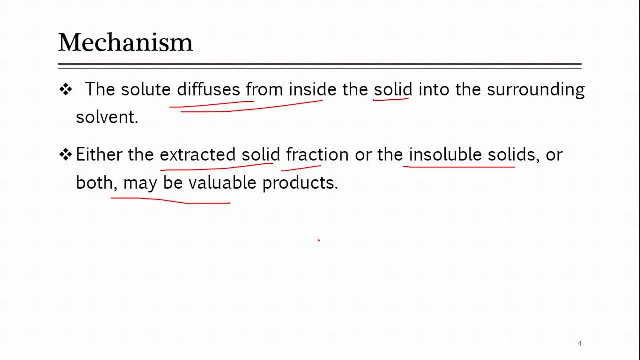 But that extracted stuff which is now part of water, that is of use, which you drink. So it depends on the application. either both are mean of your use, sometime mean some. only one of those is of your use, So it depends on the application. So licking is widely used in various industries. 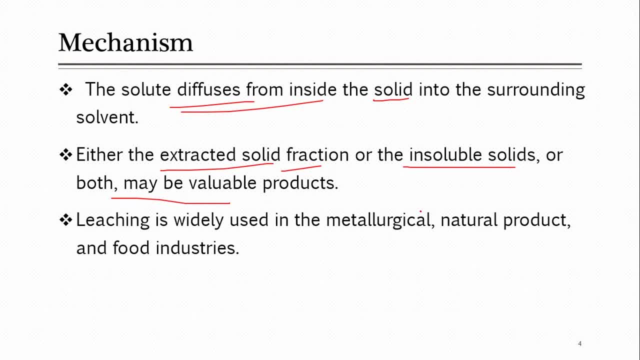 For example, for metallurgical, natural products and food industries. this is widely used technique, For example for metallurgical mean extraction of ores. you can use for the extraction of various ores. So this is metallurgical application and one major application which hopefully you are aware about. 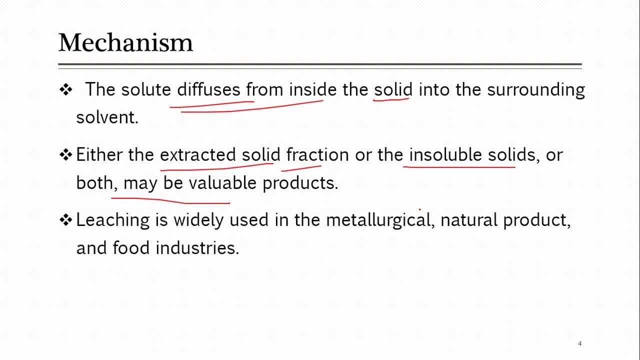 extraction of uranium, because uranium in nuclear industry is extracted from the in various mines, uranium ore. so extraction of uranium is done with the help of this technique which is called leaching. and there are various techniques for the extraction of uranium. you can go through that by Google it. so 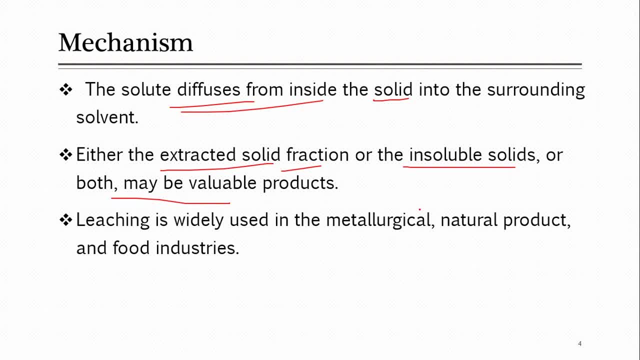 some techniques are involved, some acid. some involve some base mean you can use either alkaline solution, acidic solution to extract uranium from various ores. sometimes even in situ extraction take place, like you inject some liquid inside the main mine and you extract uranium. so there are various techniques used in the 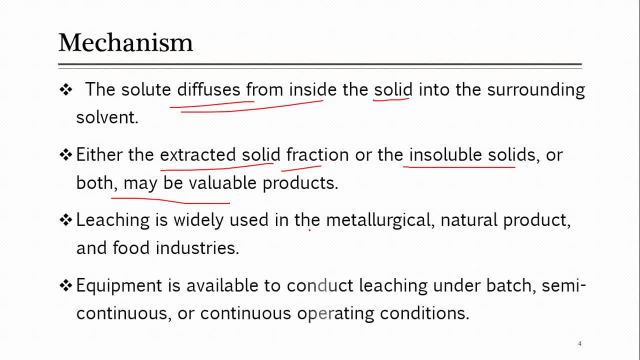 world for extraction of this uranium. that's one common example where leaching is being used, actually. and what does that liquid suppose either alkaline or acidic solution will do? it will just extract uranium from that solid ore and will come out of that, come back and we will just get it separated from that acid and liquid. that is another. 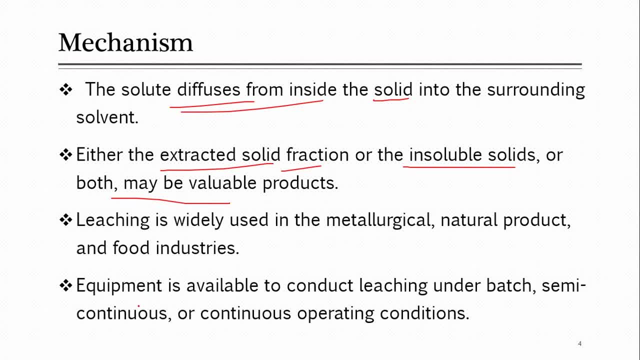 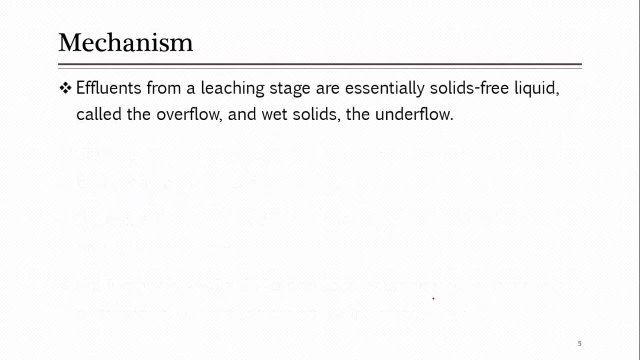 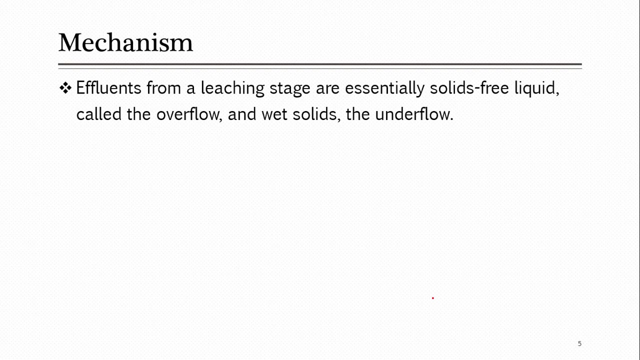 like later process, separation process, So equipments are available- mean for this leaching: either batch equipments, semi continuous or continuous operating. all type of various equipments are used based on the application in various industries. So effluents from a leaching stage are essentially solid, free liquid. finally, as you look at, 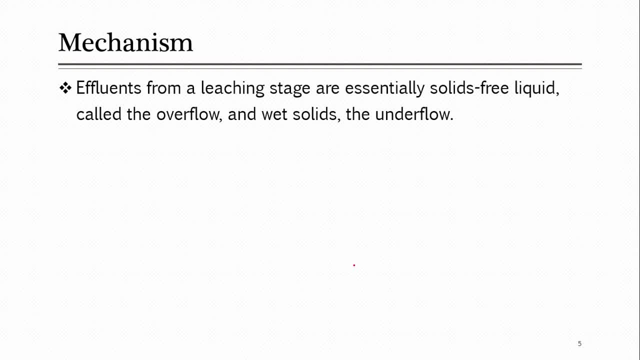 these mean, for example, tea leaves. So at the end, when you have done with the leaching, what you will get? just something solid, freeliquid, that liquid which does not contain solid, but it contains some part of the solid which is now dissolved or soluble inside this liquid. 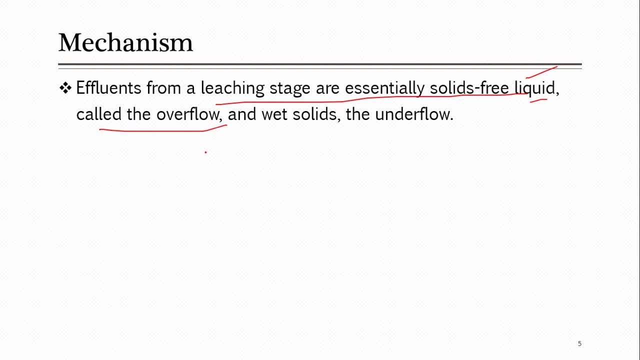 So then this is named as overflow. mean top layer, which is separated after extraction, is overflow. that's the liquid which contains some parts of the solid which are soluble, but totally there will be not like solid. due to this we call it like solid, free liquid called overflow, and there will be wet. 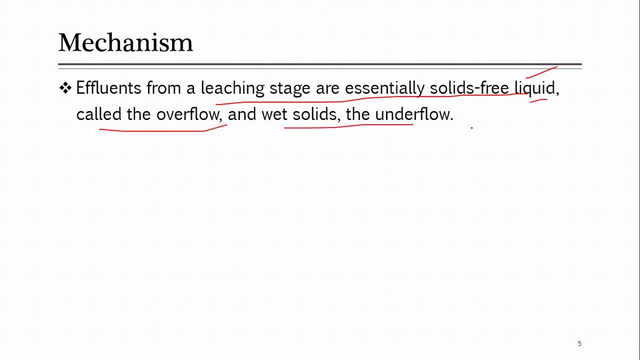 solids. they leave as an underflow. actually the solids which are leaving from that, the liquid liquid. sorry, this liquid solid extraction equipment or leaching equipment and those solid usually contain some part of the liquid. due to this he is calling, they will be like wet liquid and they flow as an underflow. overflow mean that will leave from the top of the equipment and 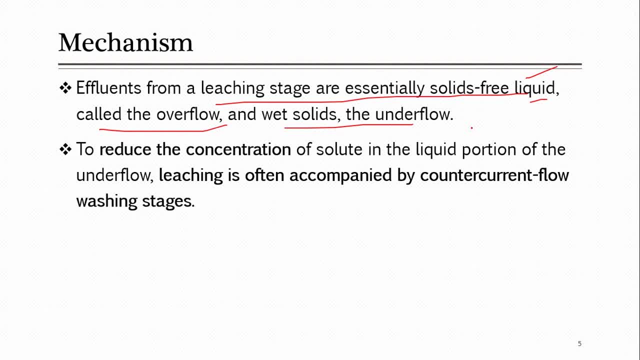 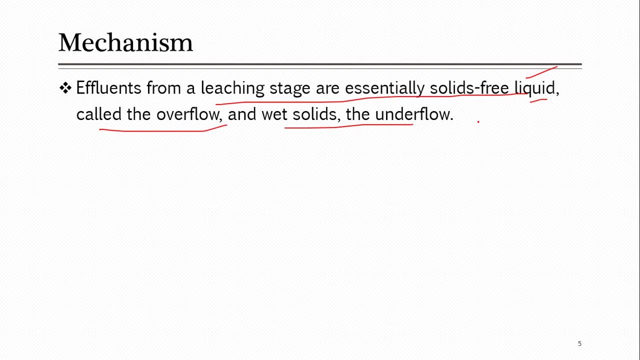 underflow will leave from the bottom of the equipment. So when you extract this in the first stage, for example, you bring in contact these solid with the liquid So that liquid extract some part of those chemical which you want to extract. So at the end, when solid is leaving from the top, that's contain some part of those extracted. 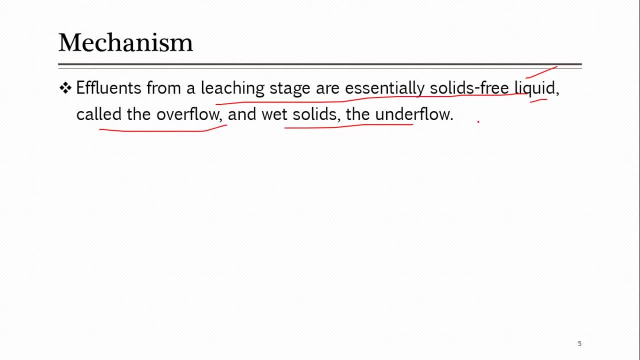 component and it is leaving as overflow, but at the same time some liquid it is leaving, as with the solid, as a wet solid. So that will also contain this liquid, will also contain some part of those extracted component, because this is a top liquid, is not separate one overall liquid. 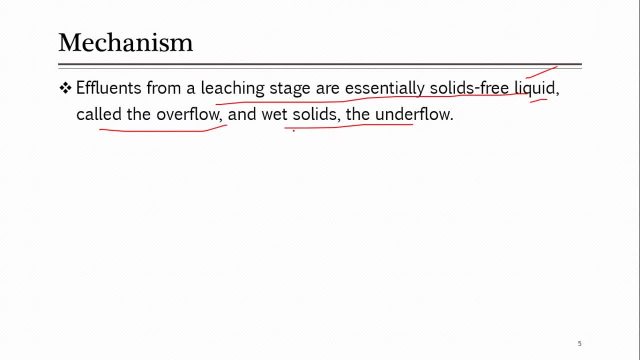 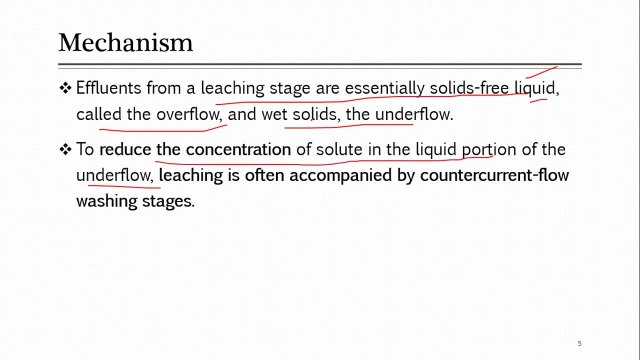 is homogeneous throughout the main equipment. So the liquid which is leaving with the solvent solids even also contain some part of those solutes, those leachants. So in order to reduce the concentration of those solute in the liquid portion of the underflow- underflow mean this- 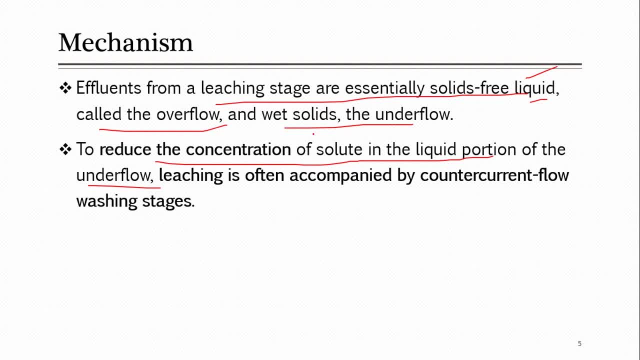 liquid which was leaving with the solid and making it wet, So that liquid will contain some part of this solute. So in order to reduce that concentration, leaching is often accompanied by a counter flow washing stages. So sometime, this is not only one stage and most of the 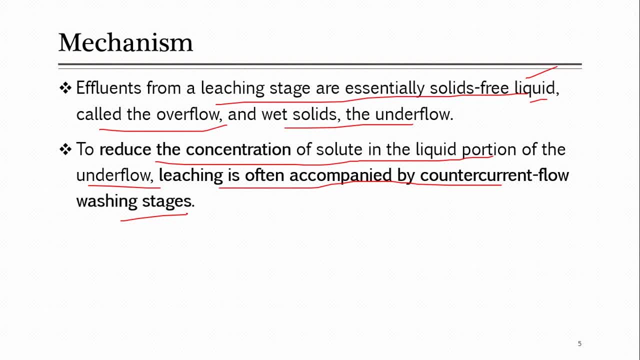 time. this is not only one stage, you have more than one stages. I will give you the example of this. for example, you dip the tea bag in the hot water. you just mix it for some time, or give it some time, So that some part of that tea is extracted to your water. Now, after 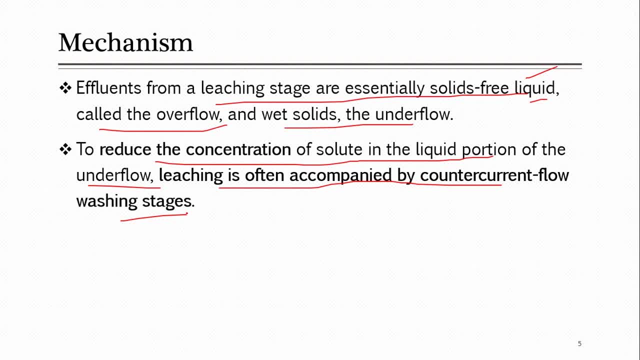 sometime you just take away this tea bag. So when you are taking away this tea bag, you most of the time you see you used to sukis that I mean tea bag with the help of spoon. So why you squeeze? actually you are just removing the water, which was part of this. 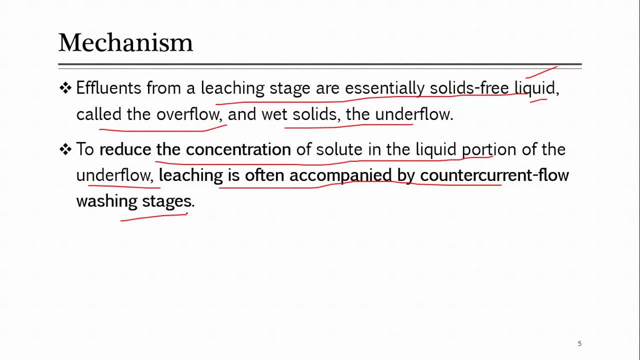 and that water will also contain some parts of this tea which you want to drink. So that is the- I mean this phenomena of counter current. somehow you can make it like similar, that is something counter current washing. Later on in this lecture we will discuss how these counter current washing. 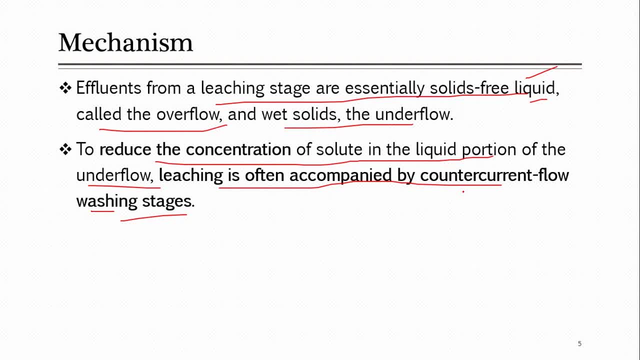 stages take place. but, for example, to understand here- just I mean keep this in mind- like these washing stages are somehow something similar, like what we do here in like squeezing of this tea bag when we are taking away it from hot water So so that we can recover maximum liquid part, as 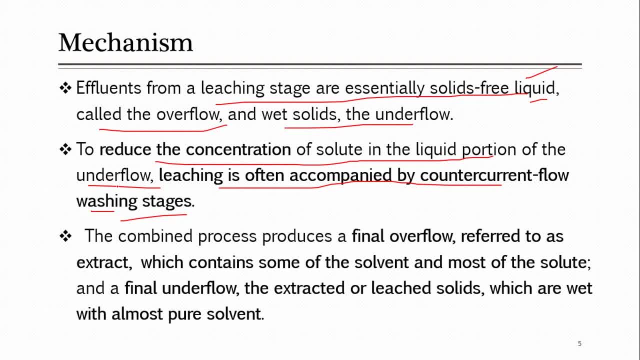 well as that solute which was part of the liquid. So the combined process overall, like you, will have leaching stage and then washing stages if there are number of stages. So at the end combined process produce final overflow referred to as extract. 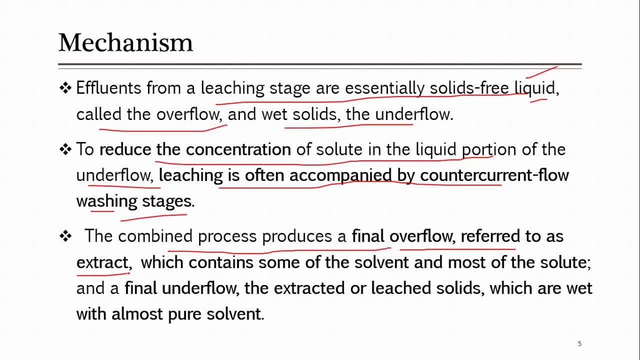 Mean When you have more than one stage is definitely this overflow will take place from one stage and it will then go to the next stage and then it move and jump to the next stage and so on, So at the end when it leave from the last stage. So it is called like extract. 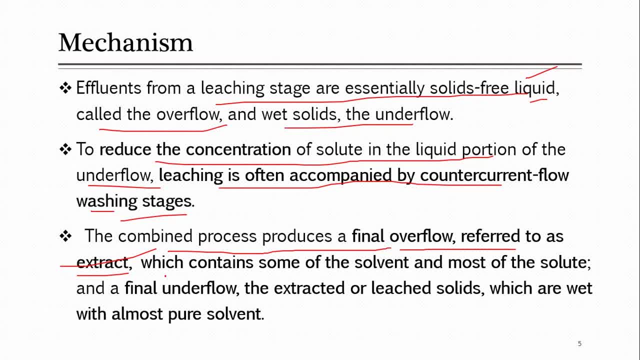 and which contain extract. you extract is that component which is overflowing and overflow. you know, overflowing is that which is the liquid or a solvent, So which contains some of the solvent and most of the solute. So this, this stream, overflowing stream, is the, your solvent containing part of the solute with it. So that is named as extract here. 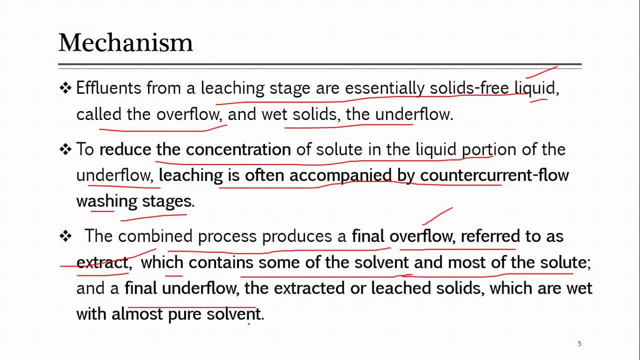 now and the final underflow. the extracted or leach solid Underflow are mostly the solids and they are like extracted or leach solid, because we have extracted some of parts of those solid and these are most of the time wet, which are wet with almost pure solvent. 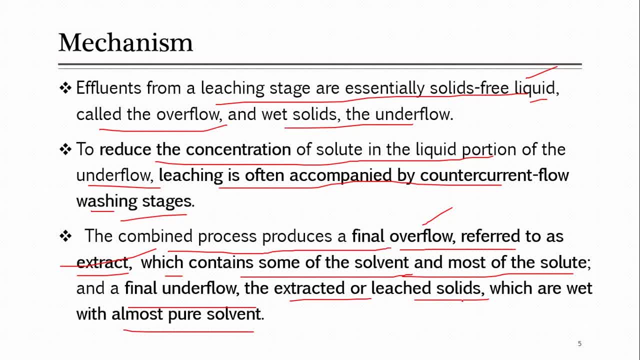 Mean That solvent Which was added. So that will be somehow part of the solid and these are the extracted solid which will be leaving from the last stage. So at the end of the day, this underflow which leave from the final stage is named as extracted or leach solid. 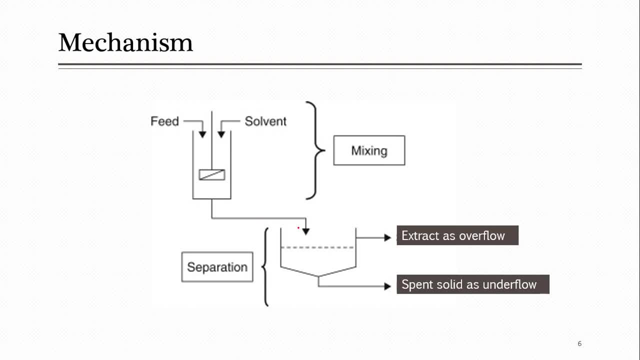 So this is the one of one stage for mean, this leaching is shown to you here. overall, you can just see that there is one stage in which mixing is taking place, and then there is separation, Why we will look at this. for example, you bring in the feed here. 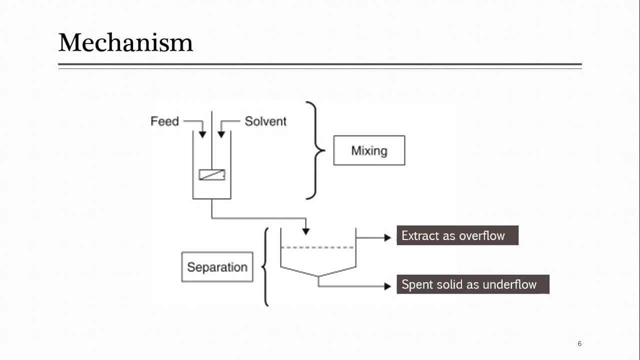 So it is the heat transfer as well as the solvent. So in this phenomena in industry for leaching you have to mix them up. So you usually go for some mixing part, some impeller type equipment to mix those. why? So that maximum mass transfer and extraction take. 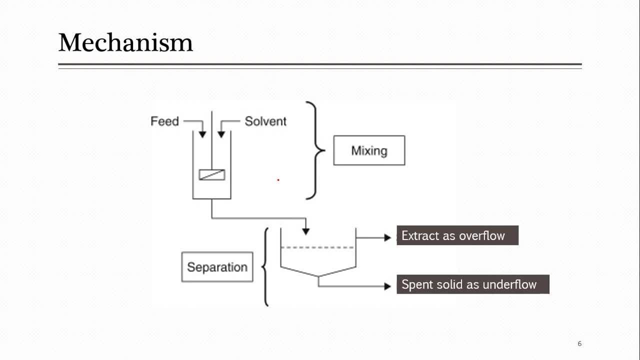 place. So after this, you just bring it or give some settling time. So for settling, you just put it to a base, and which will give separation at the end based on the gravity, Because solid will be removed. So which is that? So this is the solution. The next is: 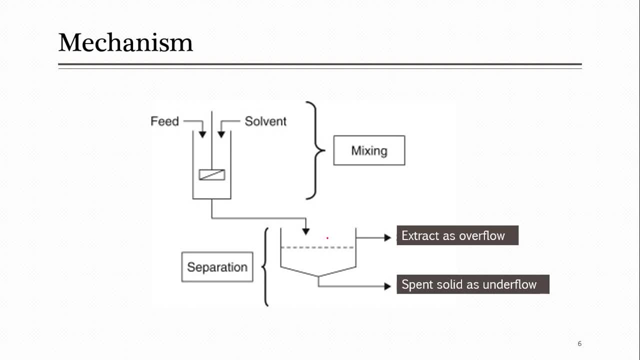 the treatment of the soil. So there are some elements there that are present here. So, as solid will settle down, it will go down and liquid will be extracted to the top. now, because the purpose of this solvent was to extract some part of the feed, this feed is in the form of solid, so 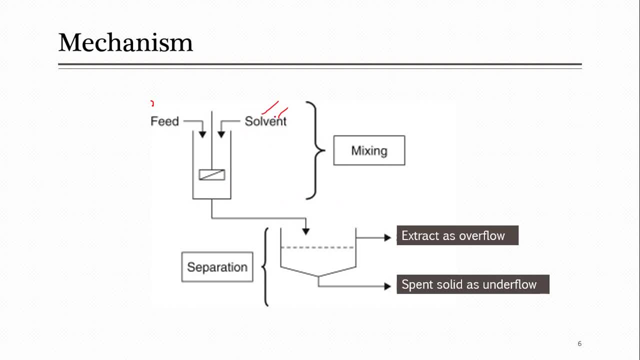 some part is extracted and becomes its main part of this solvent. so this will be like solvent as well as some solute, and thus leaving as extract as a flow overflow. as we have seen in the last slide, extract will consist of solvent as well as solute- solute that was extracted from the solid. 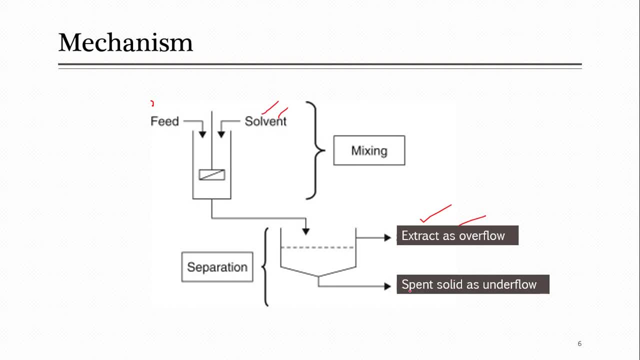 and then the bottom portion of this or under flow, that's the spent solid. spent solid, or which we called as leached solid. this is wet usually, and it contains some part of the solvent as well, as there is. I mean extracted solid, I mean, which is now deprived of those solute. this is one state. 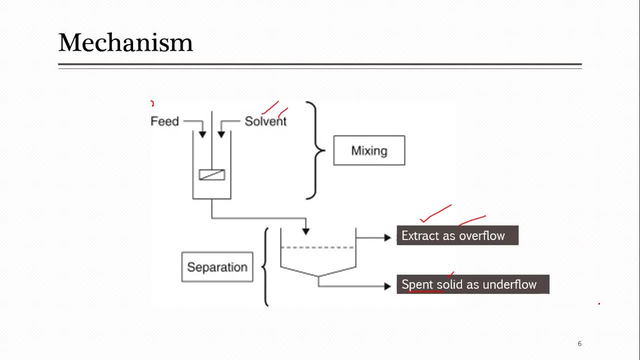 suppose you have next state, So both of these will jump to the next stage. they will again come in contact with each other and more separation actually take place and so on. actually not separation overall. we say like here: now this spent solid, which is wet solid, that will contain the liquid. now, when this liquid or solvent 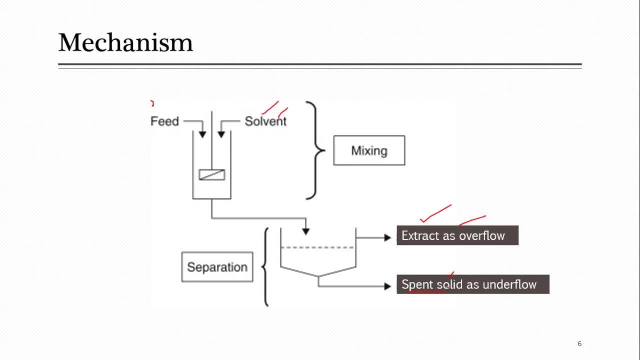 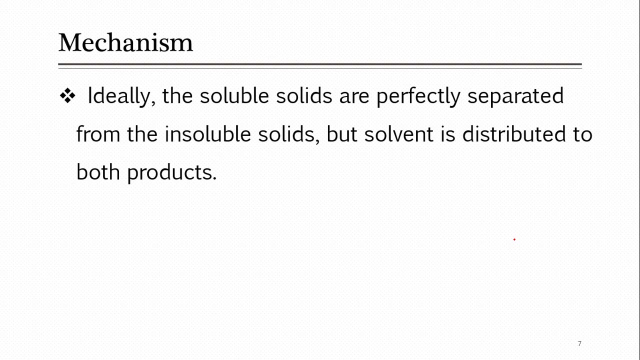 is leaving with this, that will contain some part of the solute and in order to recover that solute we will again bring them in contact and we will try to get as much extract as possible. So ideally The soluble solids are perfectly separated from the insoluble solid. mean those soluble solids, the 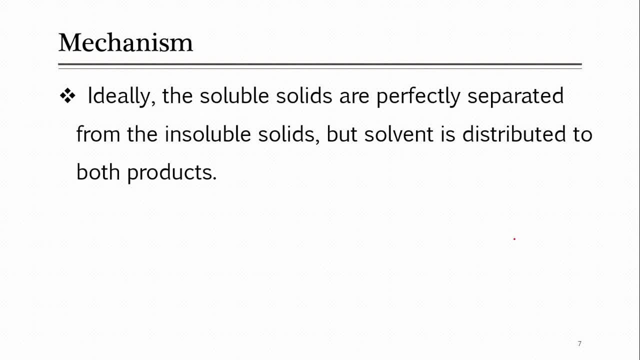 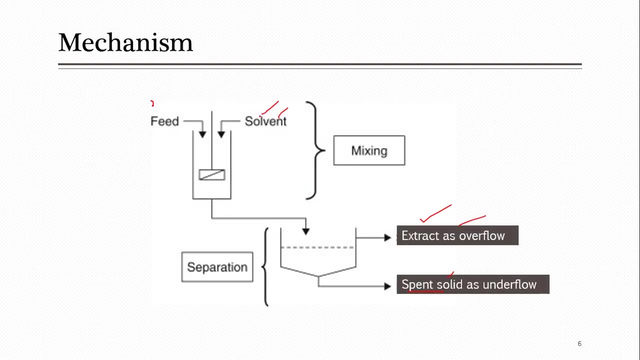 part of the solid which are soluble in the solvent. they are perfectly separated, mean you can get even 100 percent separation from the insoluble solid part, but solvent is distributed to both the products. what does this mean? like here, we have seen that the solvent which was introduced here 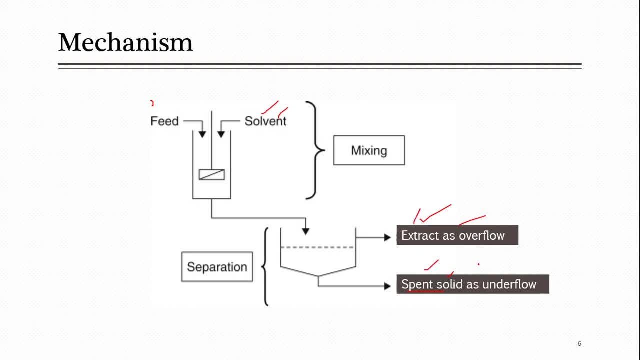 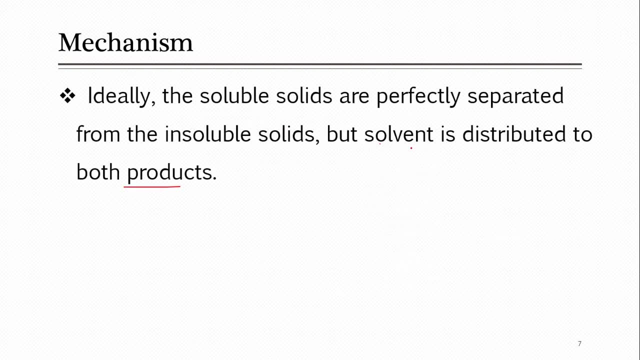 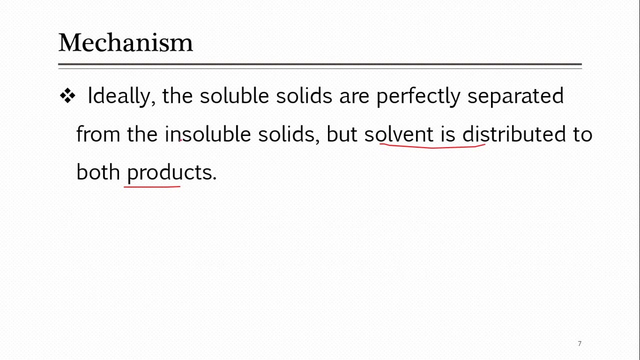 that is part of the extract. as well as this under flow Stream as well as overflow stream, so that is actually is naming it here like that. distributed to both products mean overflow and as well as in a under flow, it is distributed among both, while under flow. 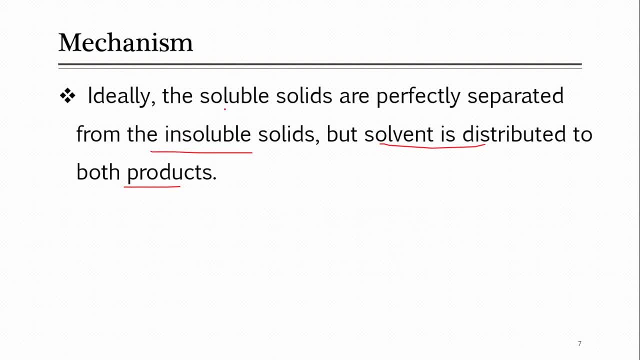 will contain most of the insoluble solid, the all of the insoluble solid, even and top stream will contain. our overflow will contain most of the soluble solid, but some will also be part of this mean under flow stream. Therefore, At the end of the day, 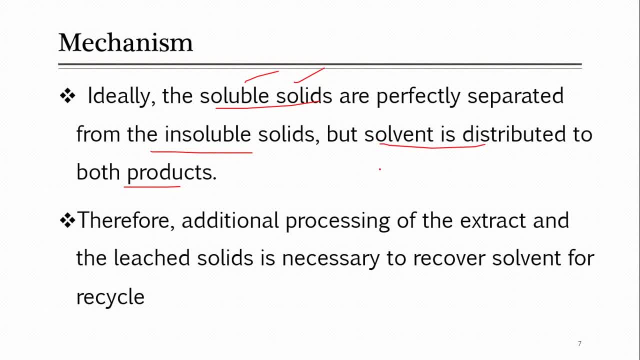 Now the solvent is usually expensive and you have to recover it. it is not like wasted. so there you will have another equipment in which, at the end, you will just separate the solvent from both of these soluble as well as insoluble solid. So due to this, we say like we have additional processing of the extract and the leach solid. 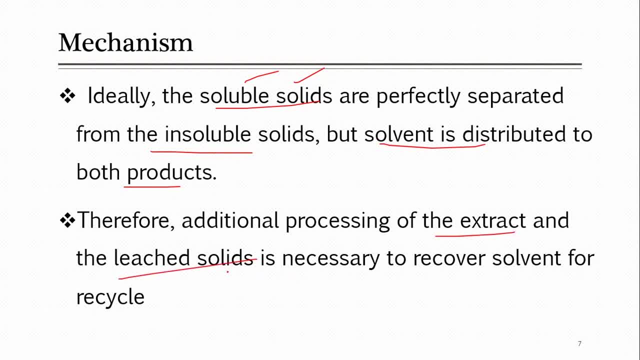 extract, which was the top layer, and the leach solid, which was the bottom layer, as under flow. So they go Necessarily. I mean for some necessary processing to recover solvent to be recycled. So this phenomenon takes place: you have to recover your solvent. 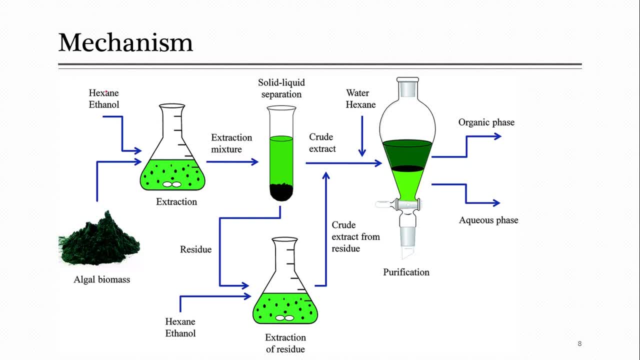 For example, here you can see, like we have a hexane ethanol, that is the solvent which is introduced with this algae biomass. So you just bring them in contact and when you are bringing, you are extracting here. Here stirring is taking place. this is the sign of stirrer. 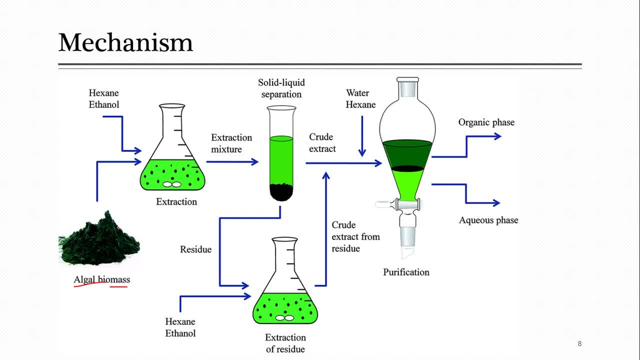 So just after stirring You will extract some particles. So you will extract some particles, So you will extract some part of this main biomass that is transferred to the hexane, because these contain usually the oils which are extracted. So those will be extracted to these main hydrocarbon, hexane, ethanol. 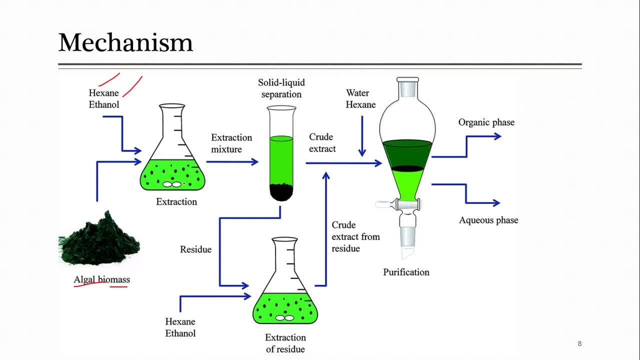 So after this, now you have to. this is the first stage, like we have seen in the last slide. first stage of extraction is mixing. So here mixing takes place. after that you have to give them some settling time. So you just bring it to some settler and here again, 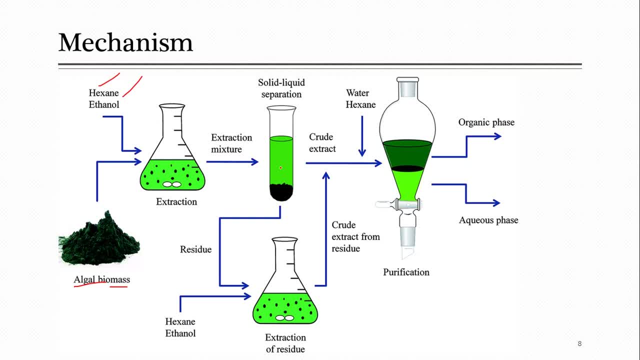 That is the, That is the base. separation always takes place easily because solid has higher density and that will settle down while liquid is at the top and then at the end of this, I mean this solid along with some liquid leave as a residue from the bottom and from top you get this. I mean crude, like here. he is naming it like crude extract. top layer is extract. 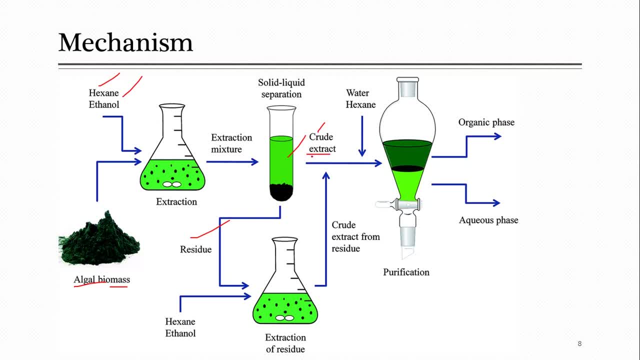 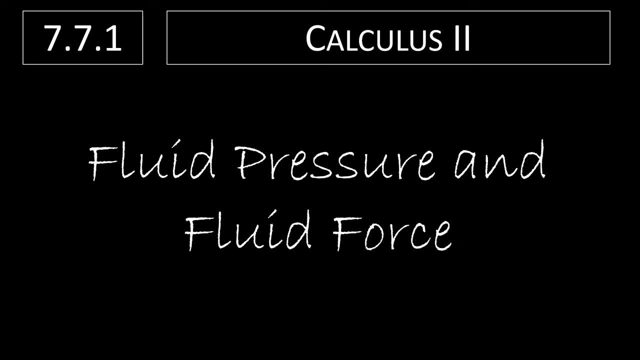 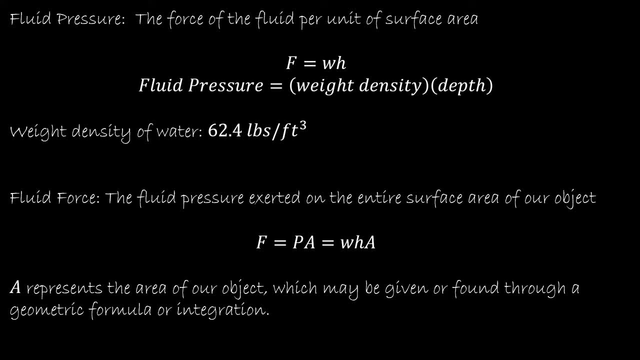 In this video we're going to take a look at fluid pressure and fluid force. Before we do any examples together, I want to talk about some of the concepts and formulas that we'll use. So the first concept is that of fluid pressure, and you should be familiar. 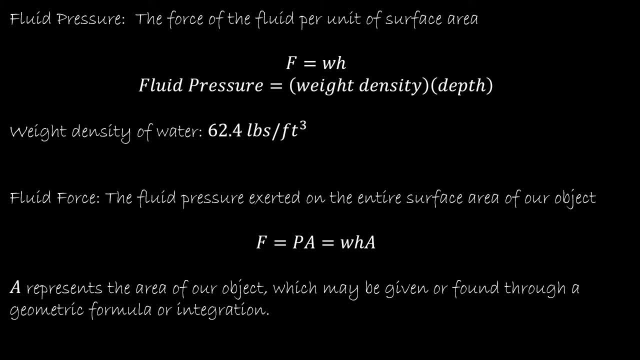 with this. if you've ever gone swimming or gone scuba diving or anything like that, We know that the deeper you get into the water, the more pressure you're going to feel. Same thing if you've been on an airplane: Obviously there's pressure. That's what makes your ears pop. 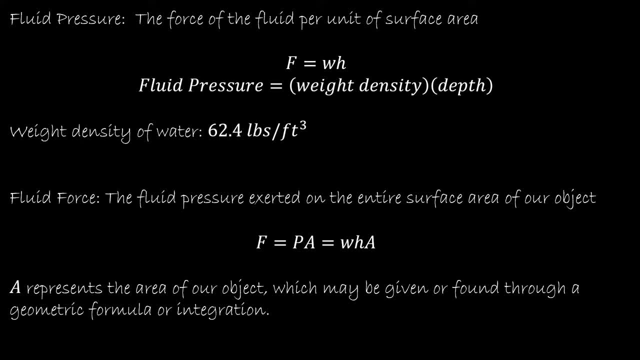 And so that's what we're talking about here. We're talking about fluid pressure. so the pressure of fluid And that fluid pressure is found just by taking the weight density of the fluid, which of course varies by fluid. We're most often going to use water, which is 62.4 pounds per 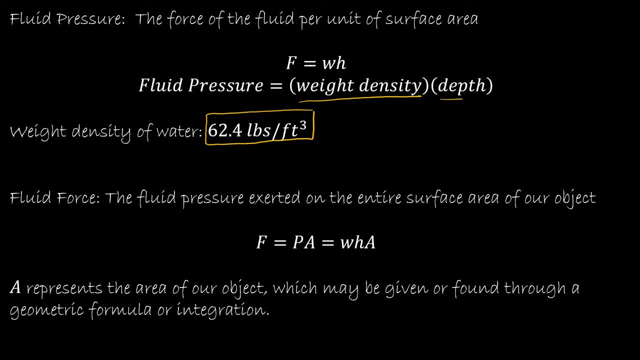 cubic foot, The weight density multiplied by the depth of the object. Now the depth is where things are going to change. The depth of the object is going to change depending on the surface. So the depth of the object is going to change depending on the surface And the depth.